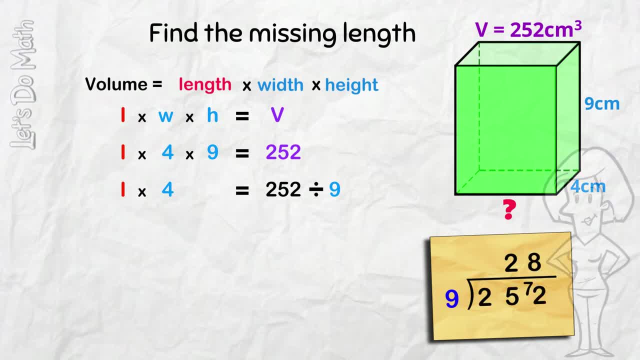 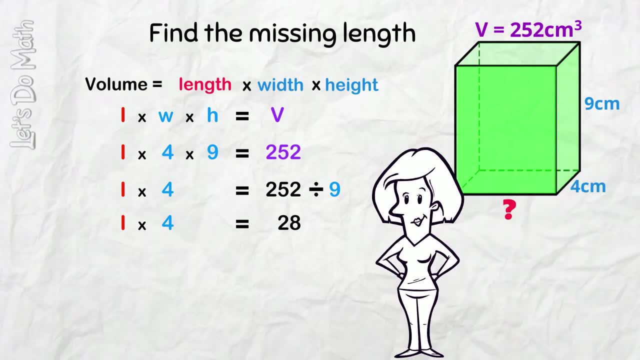 8 x 9 is 72. 28.. Now we've got L times 4 is 28.. You can probably jump to the value of L right now, But hang on, We want all the marks available right. So we finish the process and show the development line by line. 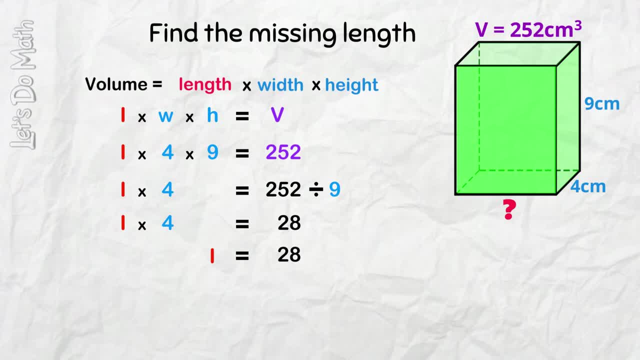 So we finish the process and show the development line by line. So we finish the process and show the development line by line. So the length is 28 divided by 4.. And of course the length is 7 cm, because 4 x 7 is 28.. 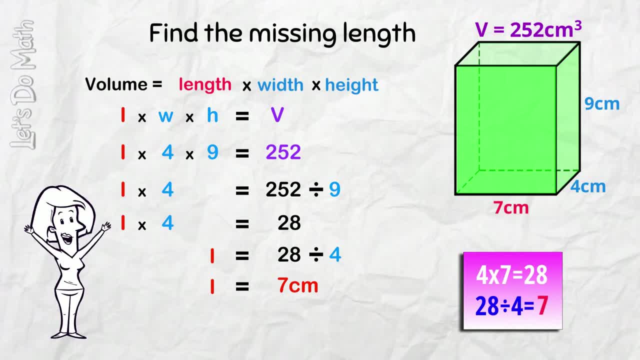 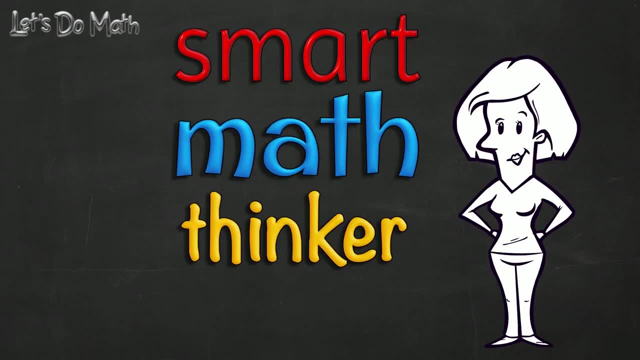 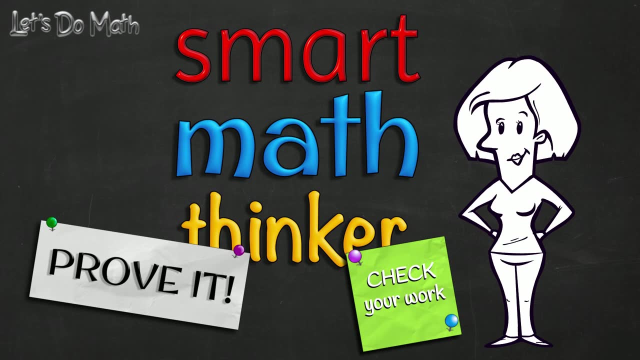 So 28 divided by 4 is 7.. But we didn't rush to it. We showed every step And, of course, being the smart math thinker that you are, you then prove it. You check your work. Do it, because this may also get you an extra mark in an exam. 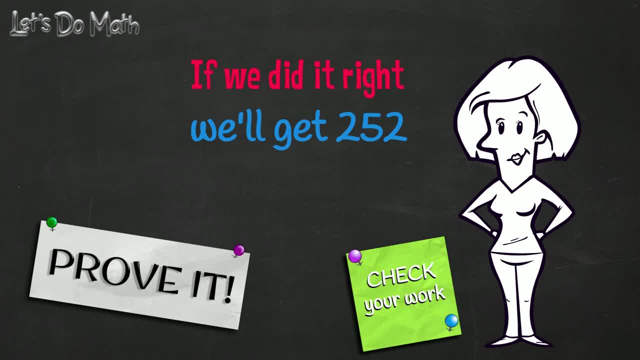 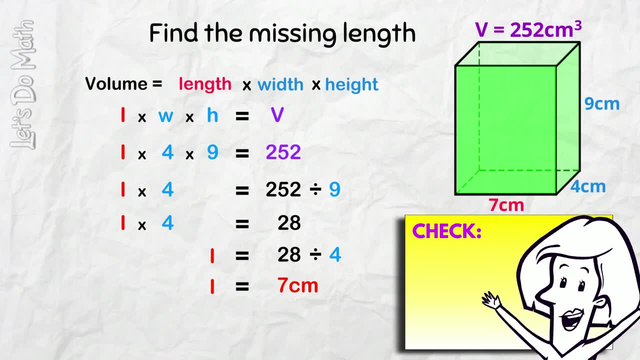 If we did it right, we'll get that volume of 252.. Set up a note to show that you're checking your own work. Teachers and examiners love this stuff. L x width, x height equals volume. 7 x 4 is 28.. 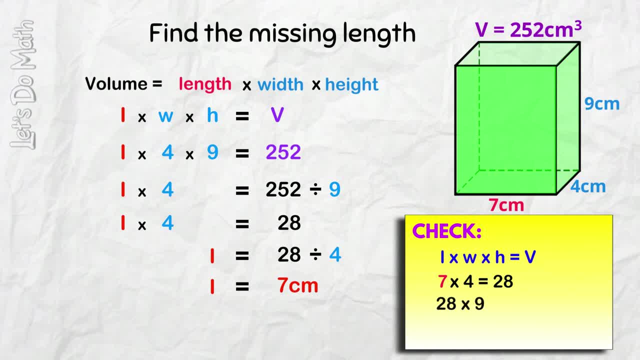 Now 28 x 9.. Write down your working out and don't erase it. 8 x 9 is 72.. 2 x 9 is 18.. And add in this 7.. That's 25252.. And that's it. 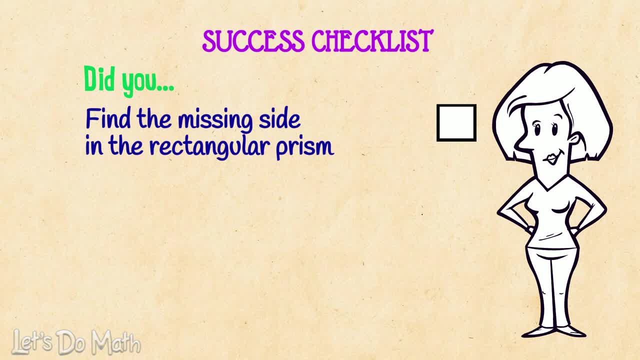 Done Aced. We found the missing side in the rectangular prism. We used the technique that gets you the extra marks And then we proved it by multiplying all the sides right back up again to the given volume. That's how you get every mark possible. 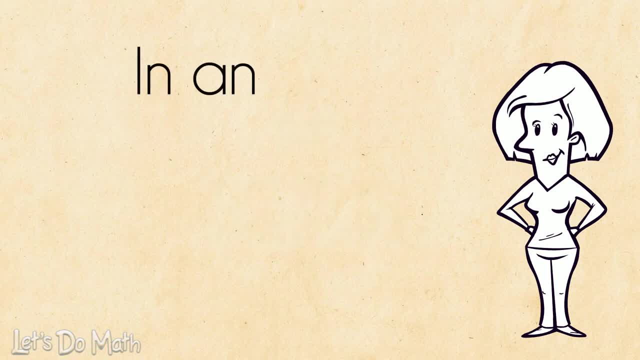 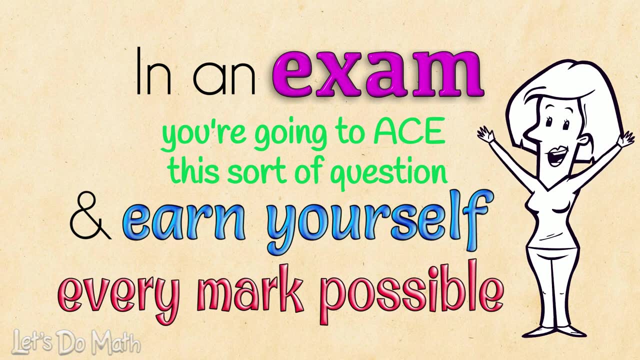 Hit the like button, Then try it for yourself And know that in an exam you're going to ace this sort of question And earn yourself every mark possible. See you soon on Let's Do Math.